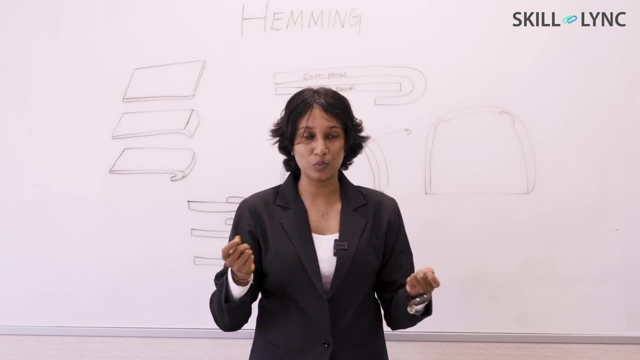 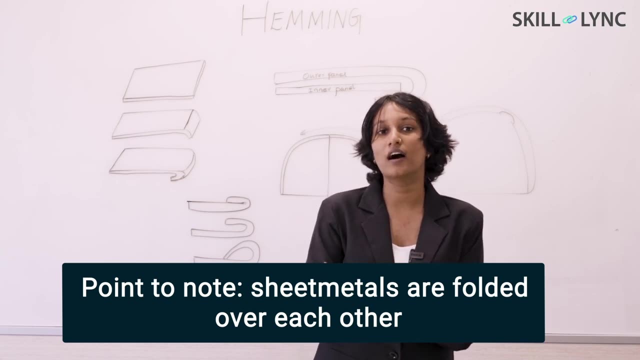 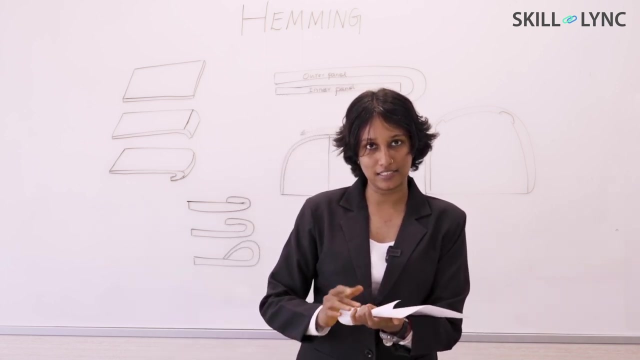 from a design perspective, Hemming is a part which we use in a sheet metal where the edges are folded over each other. That is what a hemming actually means. So when we have a sheet metal like this, the edges will be folded like this. This is what a hemming is. So what? 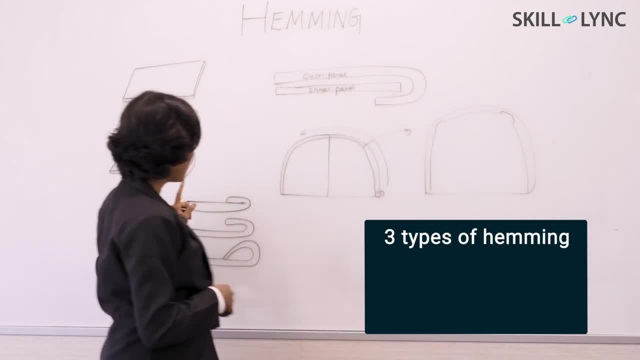 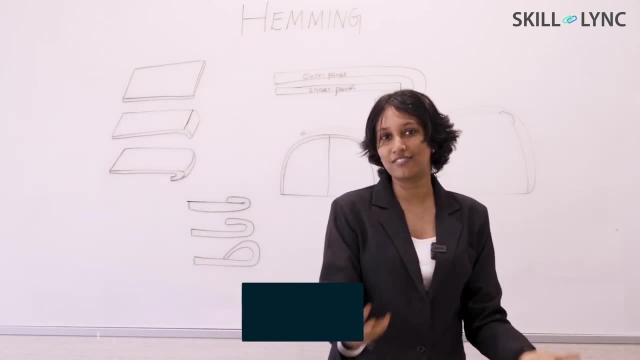 are the different kinds of hemming We have, say, for example, the flat hemming and an open hem, and this is a teardrop hem. And these are just three examples of the types of hemming which we have. and there are many more types of hemming which we can use in our day to 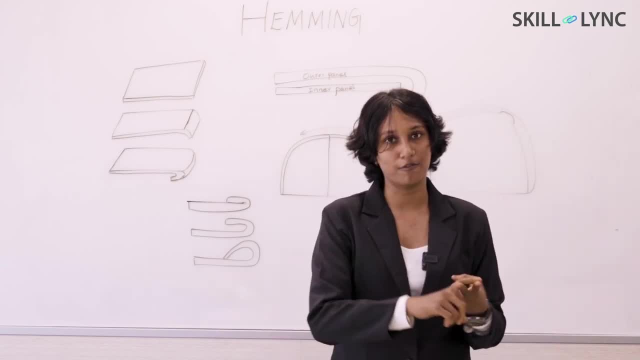 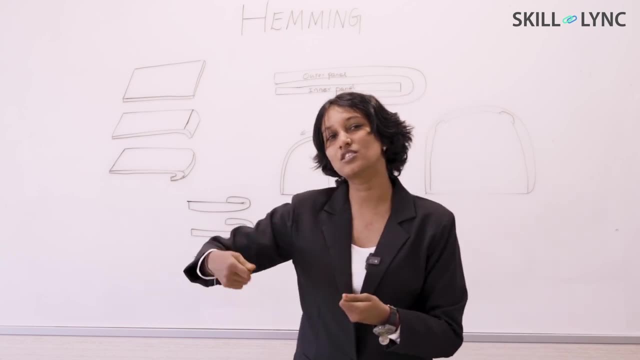 day life. But why exactly do we have to do hemming? It is, of course, a joining method. Do we have any other purposes? It serves one. When we have a sheet metal, of course the edges won't be very perfect. Just as, why do we do hemming? 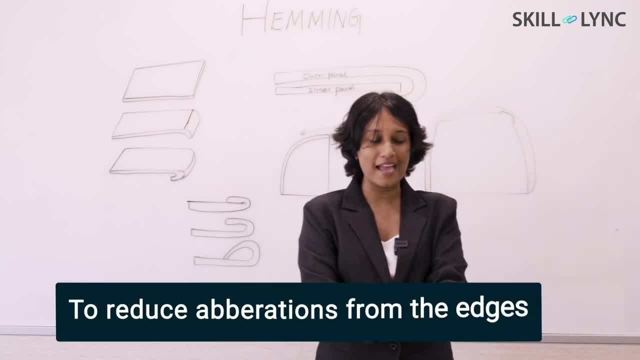 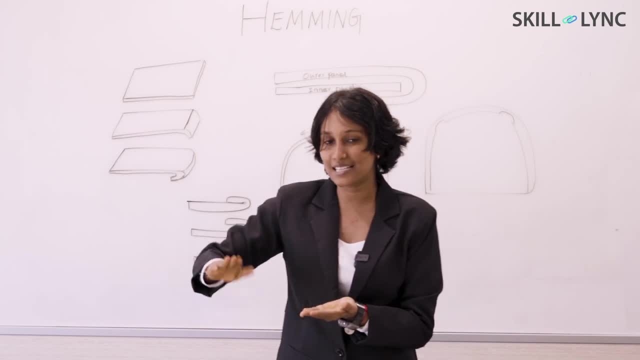 for the clothes, Because there is a possibility that the edges can be frayed. So even the edges of the sheet metal are not perfect. They are burred and there are imperfections. So to hide these imperfections we create hemming. That is the first, And second is: 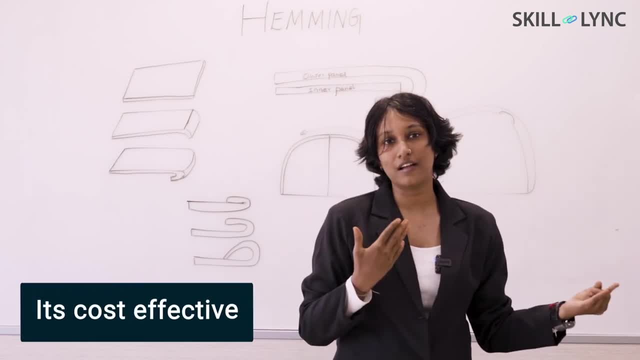 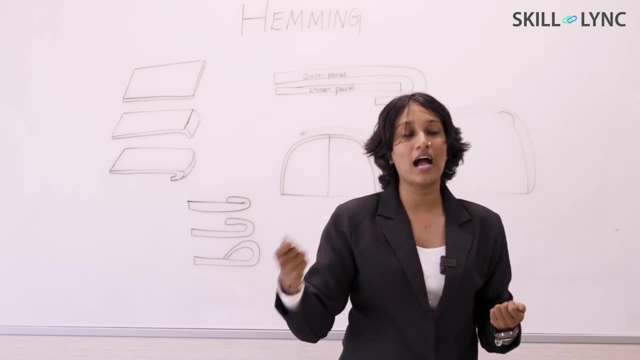 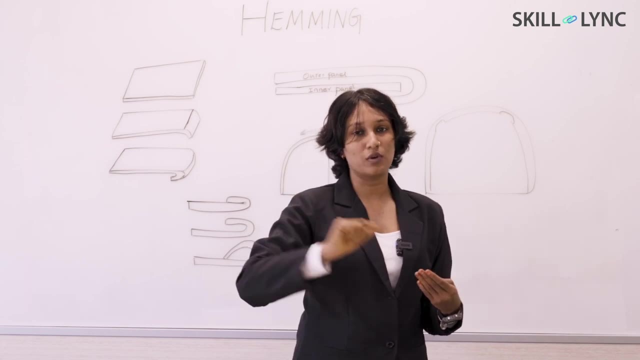 the other edge treatment method, because this is cost effective and the surface finish is good, and also to strengthen the sheet metal in the corners. The last is: when we are handling, there are certain safety parameters which we have to take into consideration, So that is one of the purposes. So these are several reasons. why do we use hemming to reinforce? 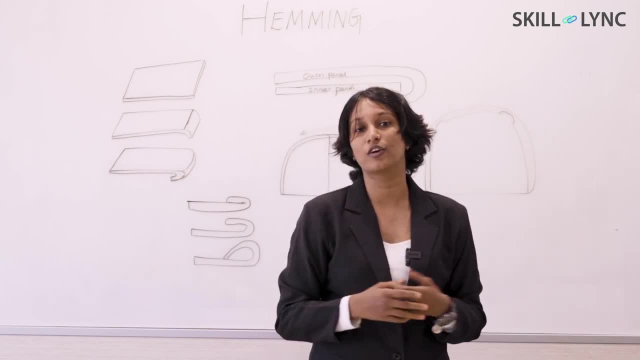 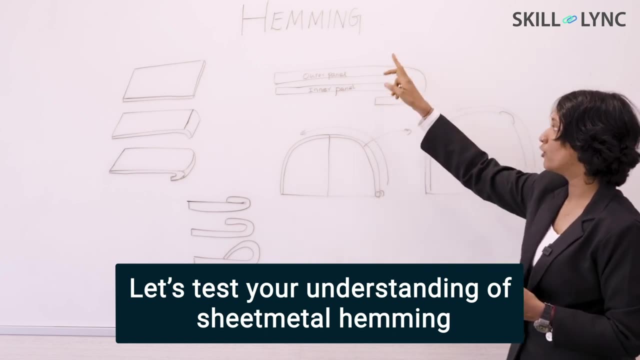 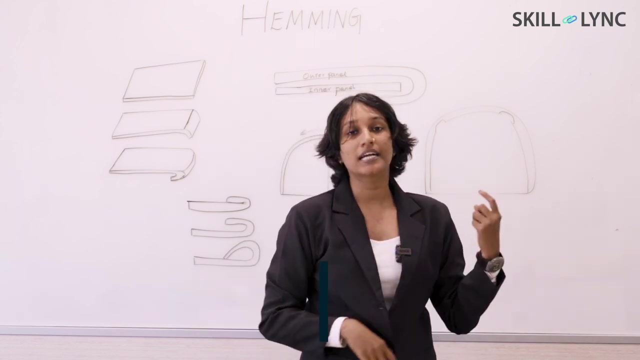 to obtain good surface finish and the aesthetic look. The hemming can be done on a single sheet metal or it can also be done on two panels. when we are going to join the two panels, How do we do this hemming? There are two major methods which we can use. One is conventional. 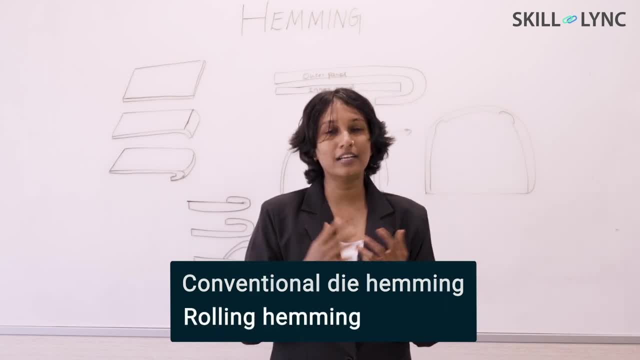 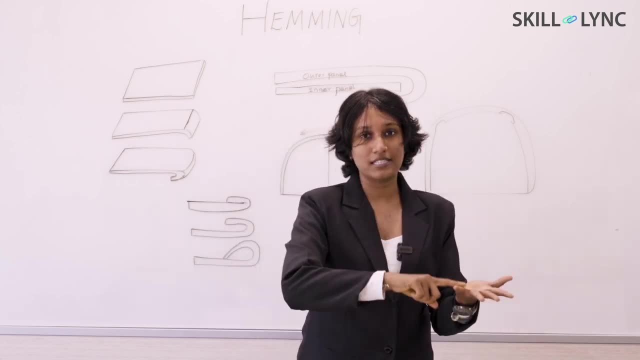 die hemming and the other is rolling hemming. So when we come with conventional die hemming, So first when we have a sheet metal, we will do different operations to it, Say, for example, drawing operations, trimming operations, several manufacturing operations. These are the primary. 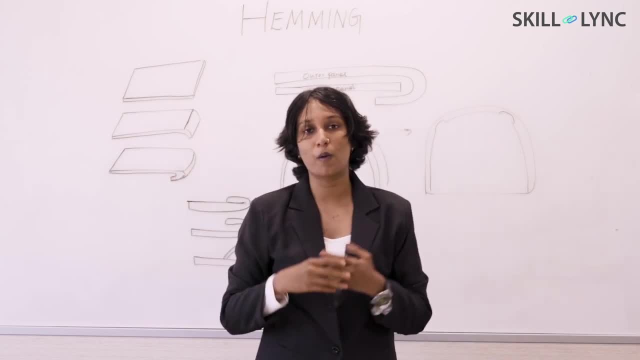 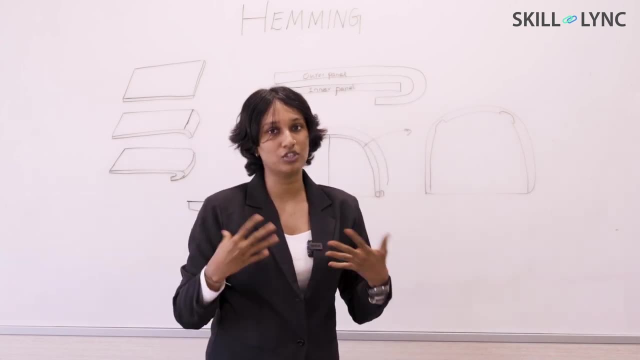 manufacturing operations. Hemming is a second type of hemming. Hemming is a secondary manufacturing operation which we use. Depending on the type of hemming we use, there can be a pre hemming and the post hemming treatments which we have to apply. 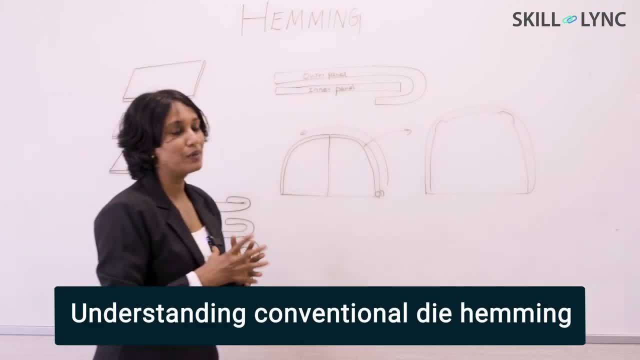 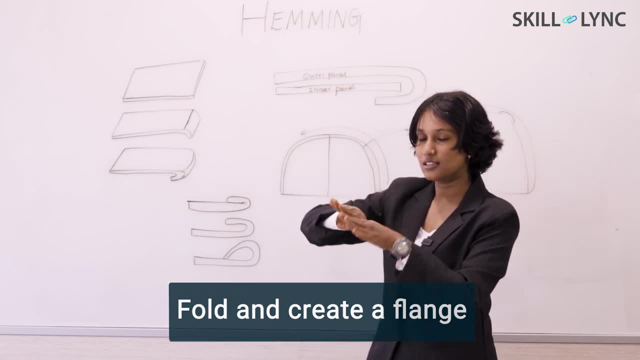 Let us first go with the conventional die hemming. With the conventional die hemming, what we do is we are just going to fold the sheet metal so that we create a flange After creating a flange. this flange can be created depending on the material that we use It. 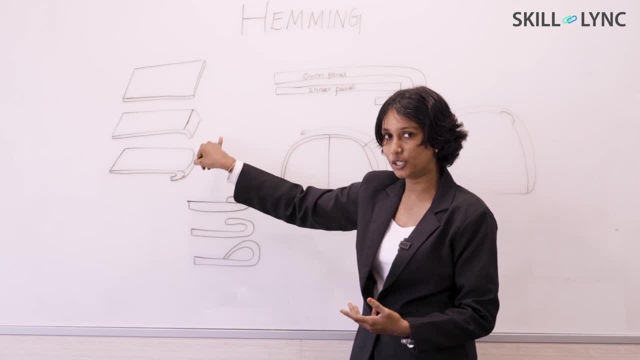 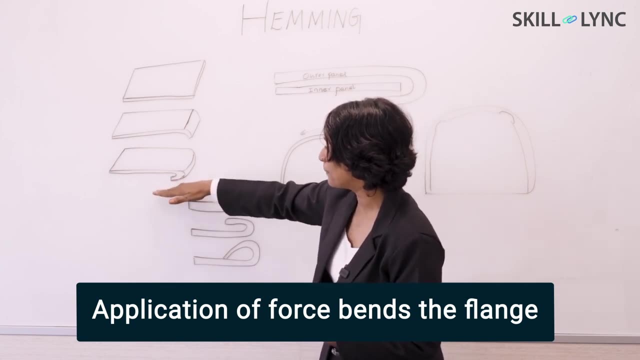 can be from 30 degree to 45 degree. So we fold it into a flange. Then after that we apply more force equally, so that this can be bent like this. So this is a flange: flange is created and after that it is bent so that the hemm is produced. This: 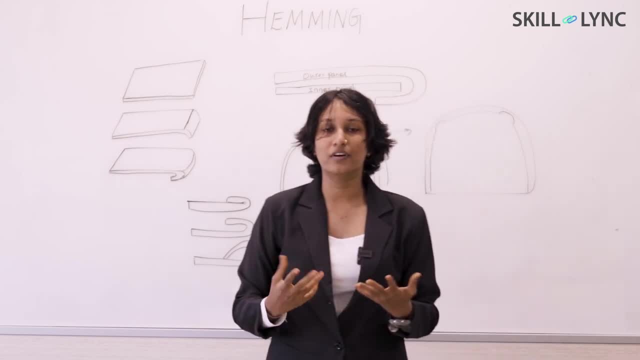 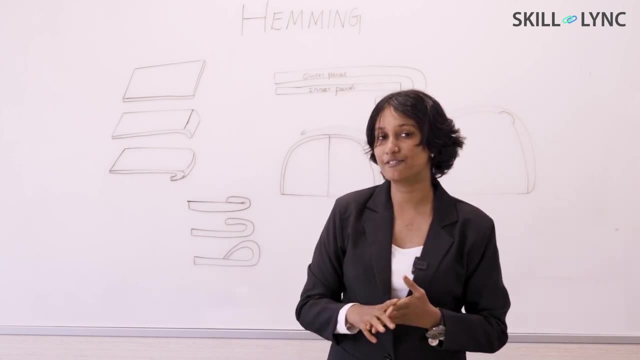 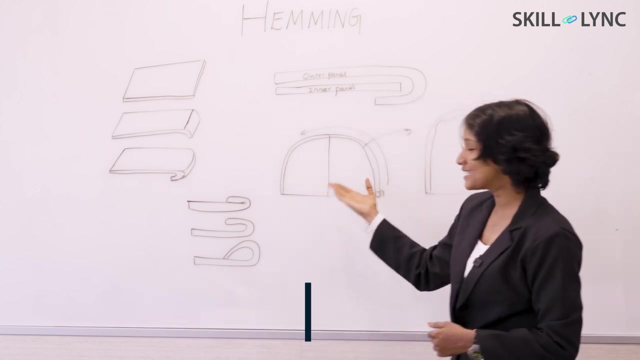 is the conventional die hemming When we do the conventional method? one is: the cost of production is high because we have to create a production layout for it specifically. But the cycle time is much lower so the product can be mass produced very quickly. The next: 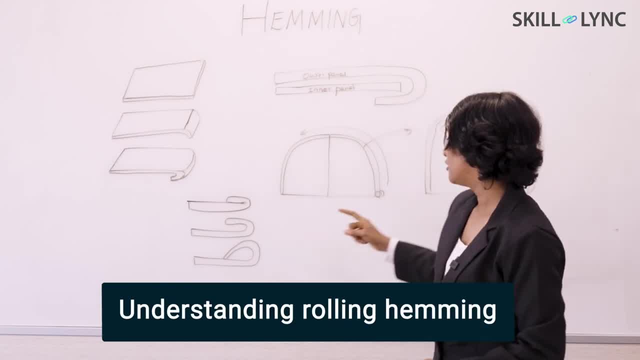 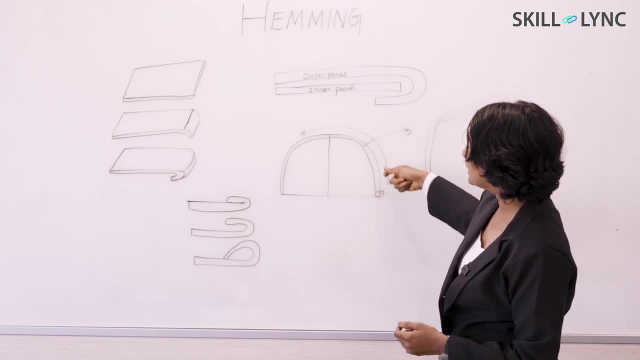 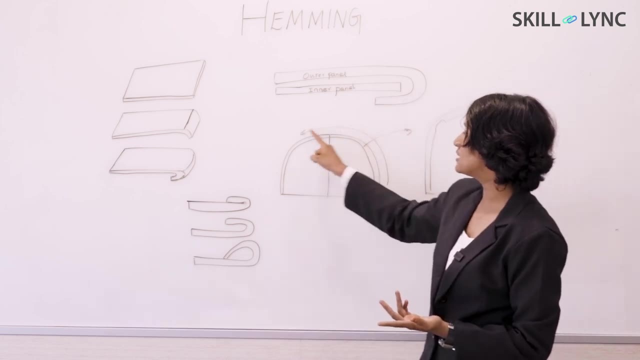 is the rolling hemming, where we use hemming rollers, where the sheet metal will be first folded into a flange, usually using a hemming tool, and then the hemming roller will incrementally fold the metal slowly, where an industrial robot can be used so that this goes in the desired. 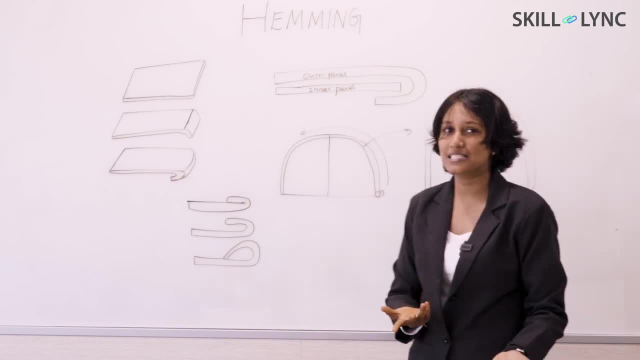 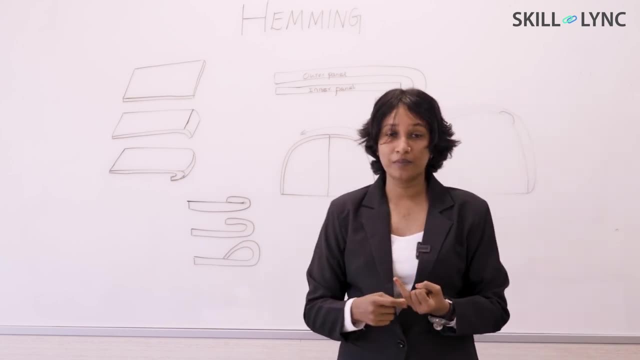 direction. When you see this method, it can be easily seen that this is definitely going to take a lot of time compared to this. So the cycle time is more, but it is very flexible where, if we are having a very complex shape where we have to perform this hemming, rolling hemming is the 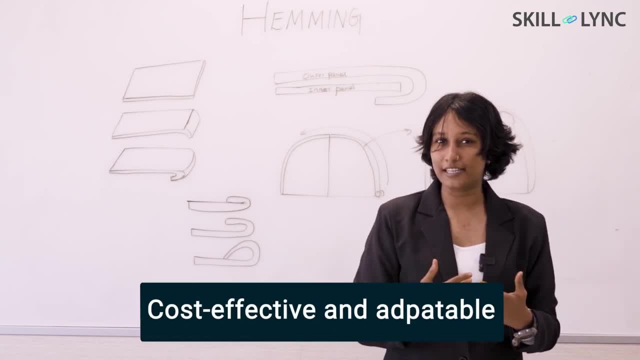 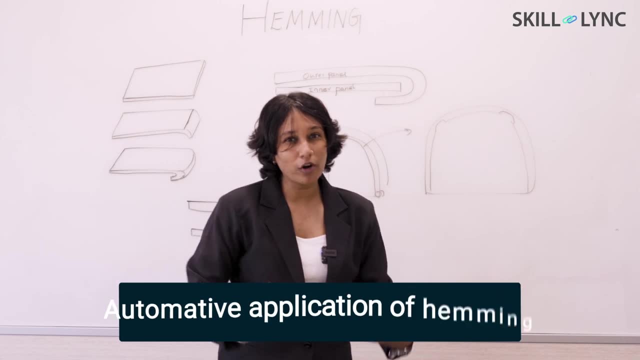 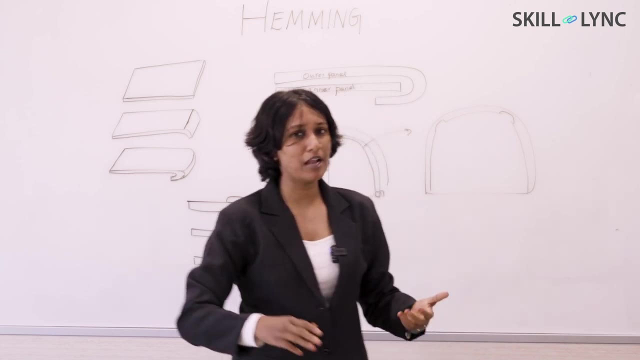 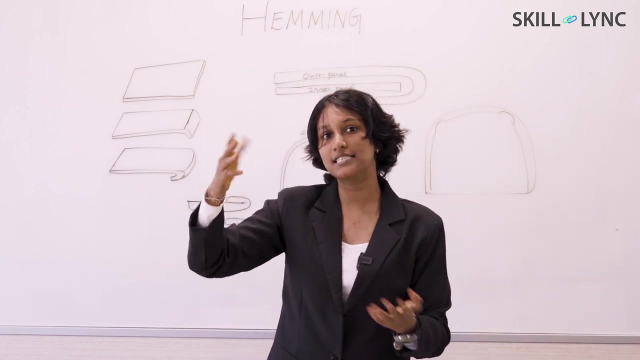 solution, So it is going to be cost effective compared to the conventional method. Now how are we going to use this in an automotive industry? that is our next focus. So in an automotive sheet metal design, say, for example, I am going to design a car's bonnet. The car's bonnet is not just what you see inside if you open your car bonnet and 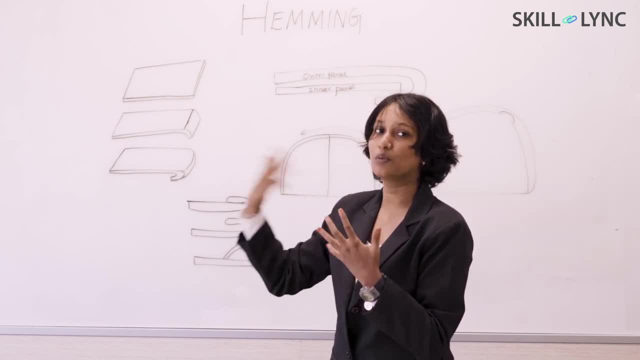 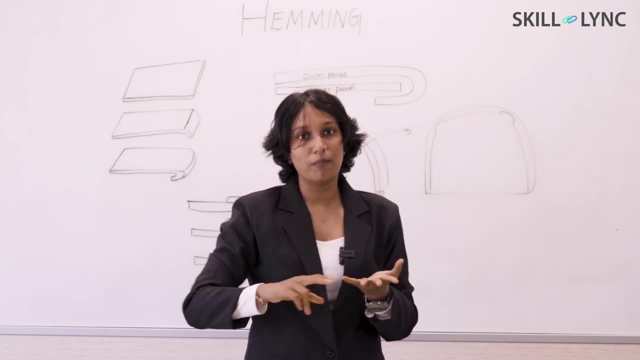 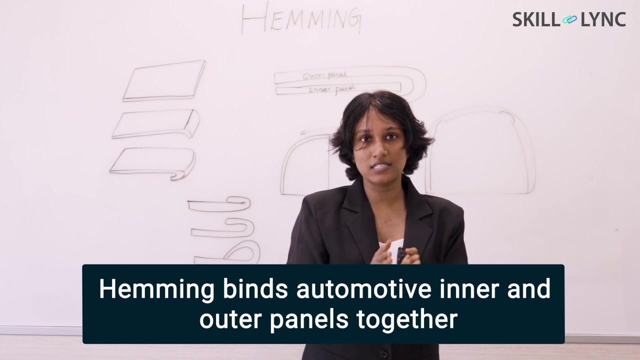 see inside. the shape that you see is not exactly what you see on the outside. that is outer panel. whatever you see inside is the inner panel. So say not only the hood, that is a bonnet, even the car's back door and the car's door have two panels attached together using a hemming operation.